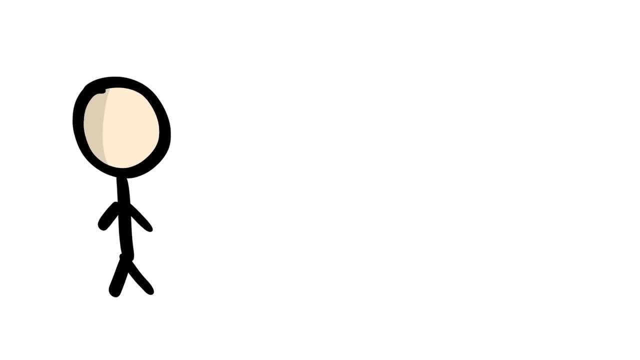 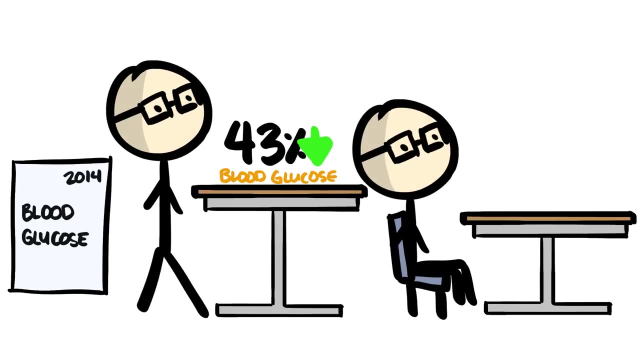 our expectations. For the most part, standing is better than sitting all day. A 2014 study did show a substantial 43% attenuation of blood glucose levels with standing versus sitting at office-desk. after subjects had lunch, People standing were also burning roughly 50 more. calories per hour. However, a 2016 study found only an 8-calorie increase. Maybe it's switched somewhere in-between. Outside of blood glucose and weight management is the development of varicose veins, the enlargement of veins in your legs and 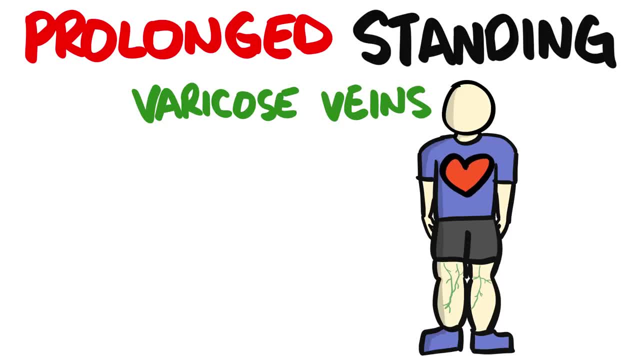 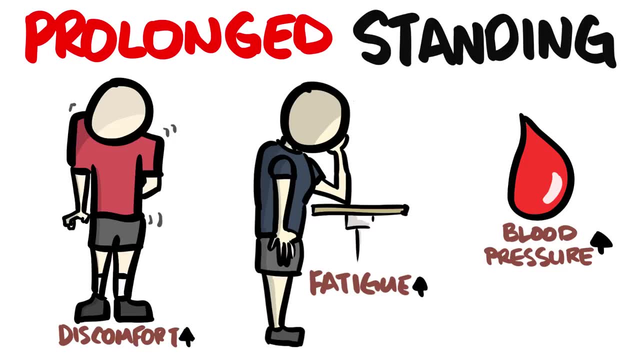 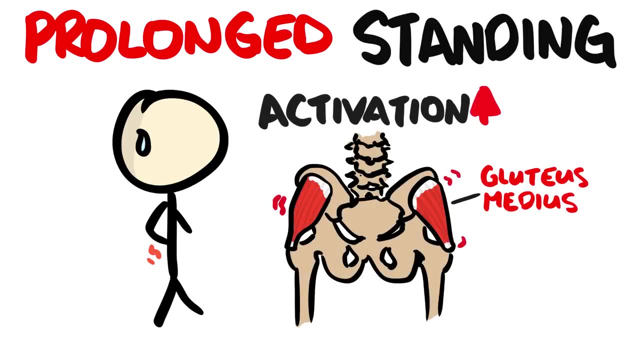 feet, making it more difficult to pump blood back to the heart. There's also reports of increased body discomfort, physical fatigue and blood pressure And, just like sitting, it can cause lower back pain, but in a different biomechanical pattern. Too much activation of your glute medius, which 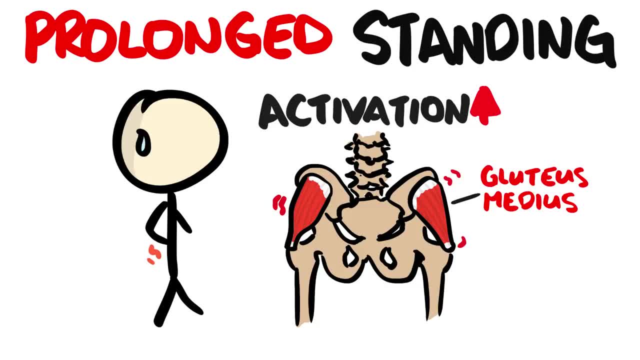 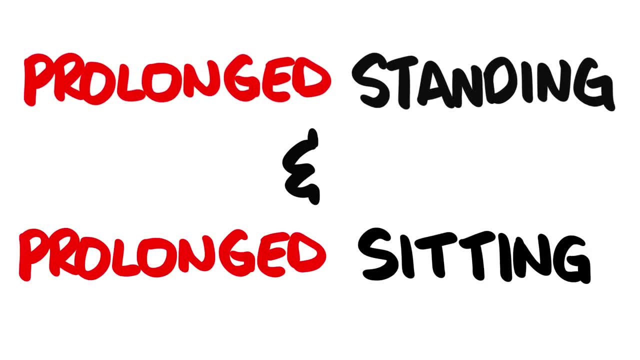 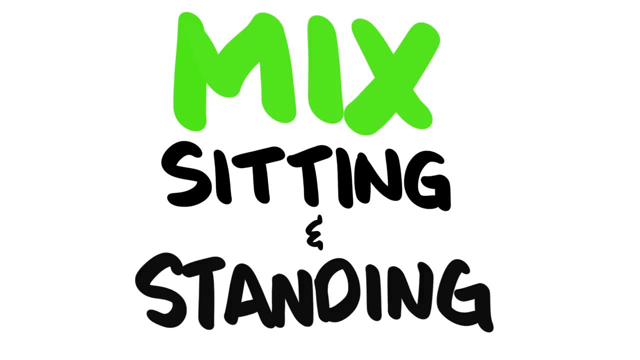 also acts on your hips and back was observed in people reporting back pain with jobs requiring prolonged standing. So if prolonged standing and prolonged sitting is bad for you, then what's the best alternative? Interestingly enough, the prevailing theory is to mix both together: The positions of sitting and 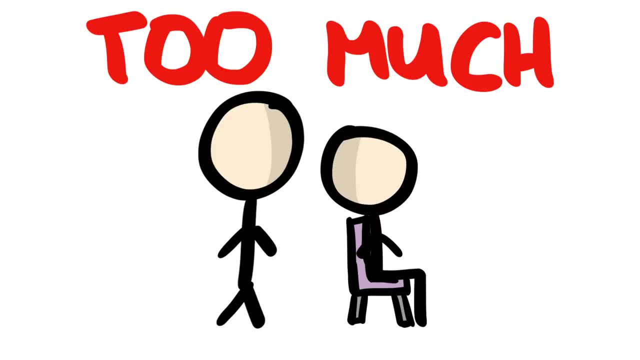 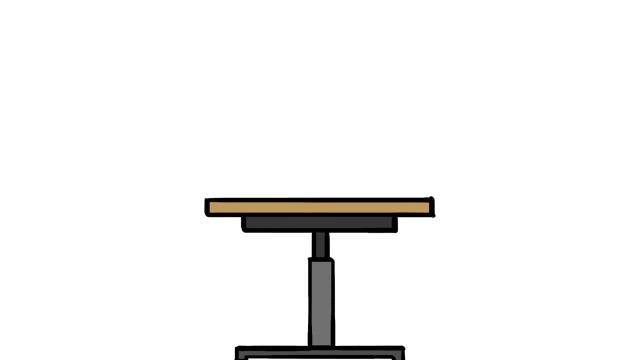 standing per se aren't the problem. It's the fact that we do them for too long. By alternating between the two, we can limit the duration of both, And that's where sit-stand desks or adjustable desks can be the best. 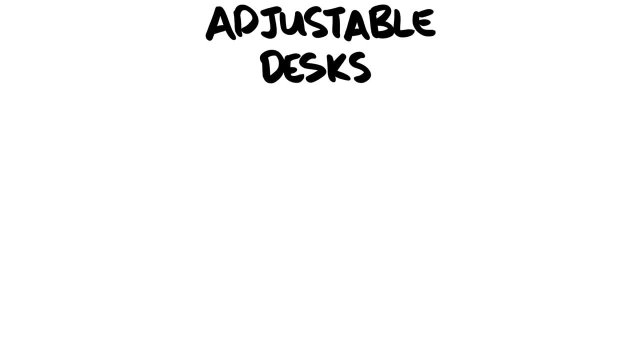 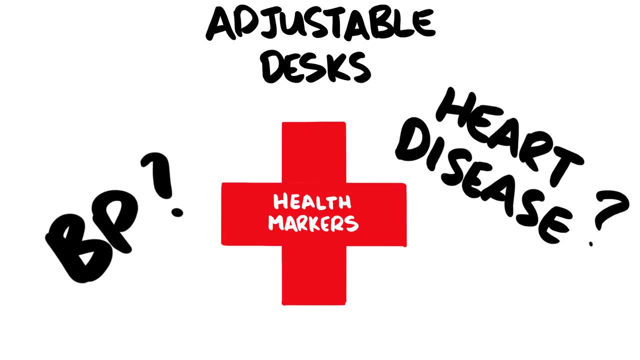 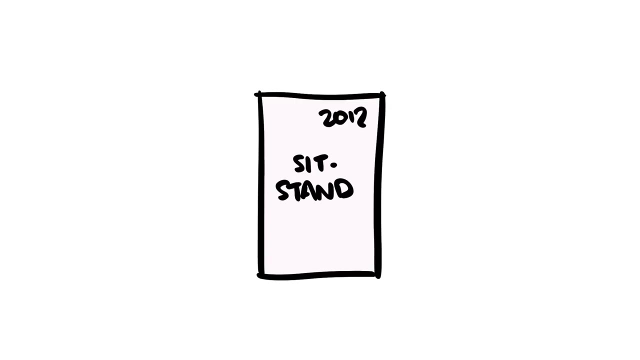 option. First, there isn't any effective research on health markers with using sit-stand desks, so it remains to be seen if using one can improve things like blood pressure or heart disease. But for many other important life aspects, adjustable desk research is quite positive. A 2012 study noted that 87% of 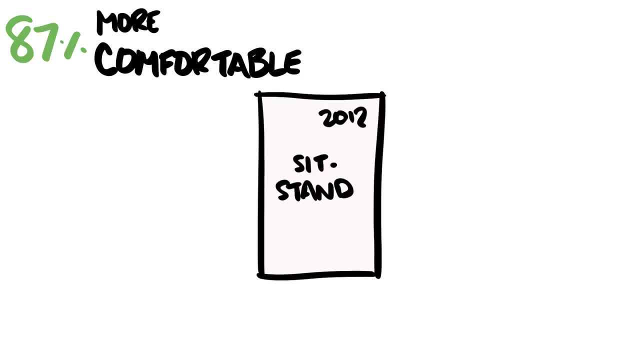 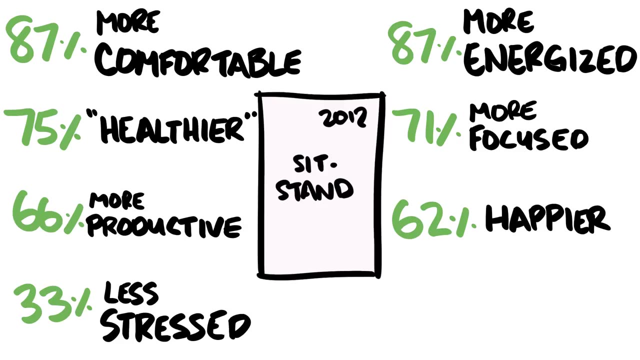 subjects. using sit-stand desks instead of sitting felt more comfortable, 87% felt more energized, 75% felt- quote- healthier, 71% felt more focused, 66% felt more productive, 62% felt happier and 33% felt less stressed. Echoing the 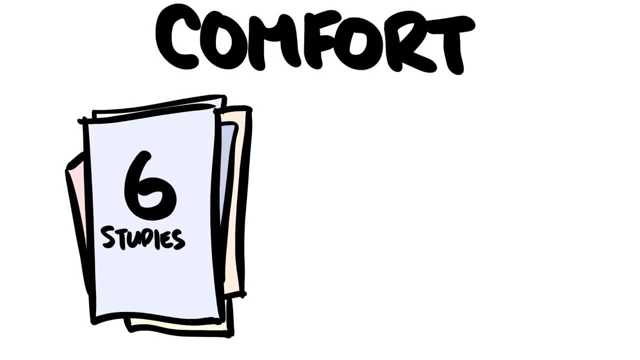 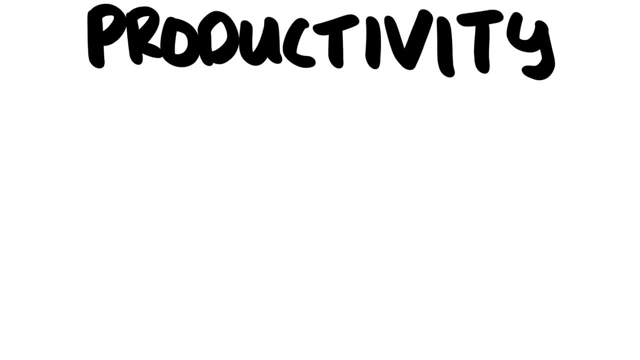 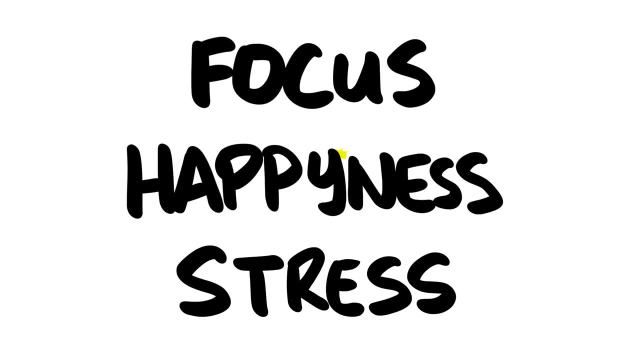 sentiments of comfort. a 2014 review found six studies indicating reductions of perceived discomfort. Productivity is a mixed bag, but only in terms of studies showing either an increase in productivity or no change at all. And certainly focus, happiness and stress is widely subjective and can be different.